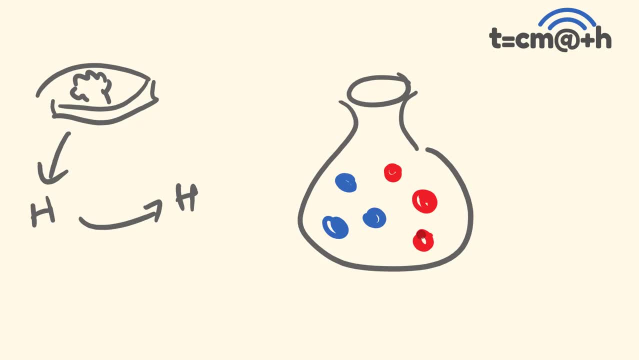 Three blue marbles and three red marbles, And what would be the probability if we were to draw out two marbles and maybe getting both of them being red? And so we're going to be looking at these types of questions. Okay, what you're going to notice with these is these probabilities occur over multiple events and are easy to work out. We're just going to keep in mind a few things In this video. we're going to be looking at some of these sort of things, So we're going to be looking at product and addition rules and probability, as well as events- how they can be independent or dependent on each other. 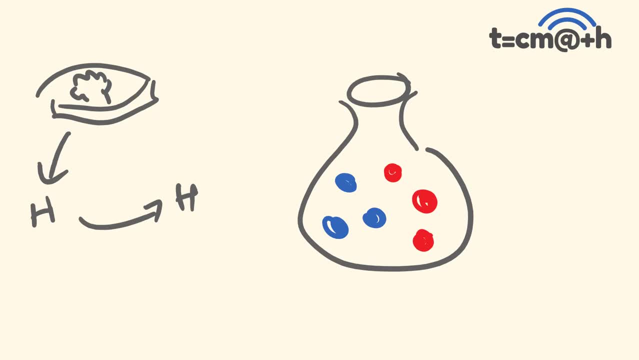 And how these affect our calculations. So let's just get on and have a look at these with a few examples. And don't forget, if you like this video, don't just sit there and lightly caress the like button. Actually, smash that like button, Smash it, Hey. and if you haven't subscribed already, please subscribe. Anyway, I'm just going to look at a few examples. 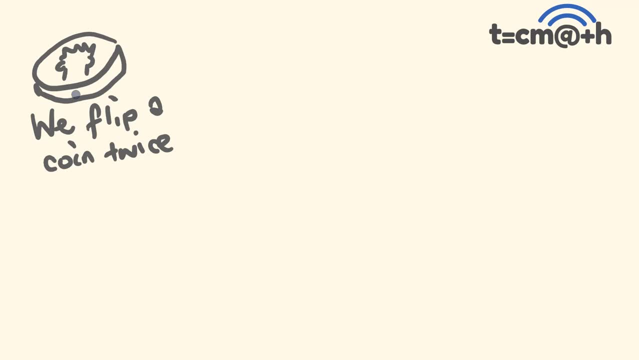 Okay, for the first example, we're going to have a look at this. We're going to be considering flipping a coin twice and just having a bit of a look about how we might work out various probabilities of outcomes that might occur. So to illustrate this, a really good way would be a tree diagram. So we have our first flip And we could get two possible outcomes: we get a head or a tail. So we get a head or a tail. This would be our first flip. We have a second flip where we have also two possible outcomes. we get, once again, a head or a tail. Or we could have got a tails first and we could get a head or a tail. 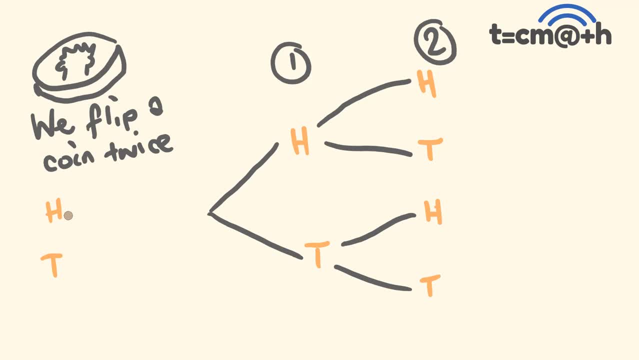 Now just a couple of things which is really important to probably get at this stage, which is this what you're going to notice: the probability of each event occurring a probability of getting a head is one in two. the probability of getting a tail is one in two. And so our first flip here: the probability of getting a head is one in two. the probability of getting a tail is one in two. we would consider a second flip. you probably notice really quickly that it's also the probability of getting a head here is a one in two. 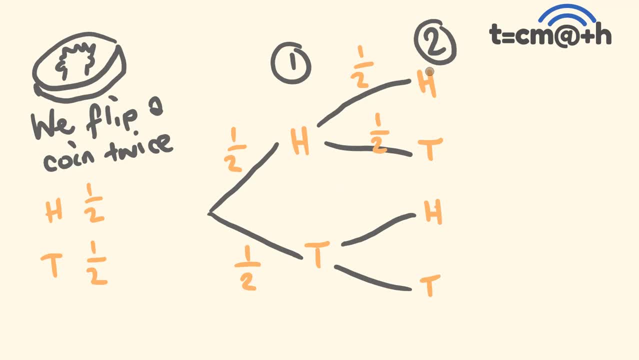 And the probability of getting a tail here is one in two. That is to say that these particular events in the second flip are independent of the first. I'm actually going to write that down. it's a really important thing to get this word here, that this is in dependent. okay, that each particular outcome or each probability is independent, or each event is independent of the other event- Okay, it's not affected by it. So we have a half chance of that. 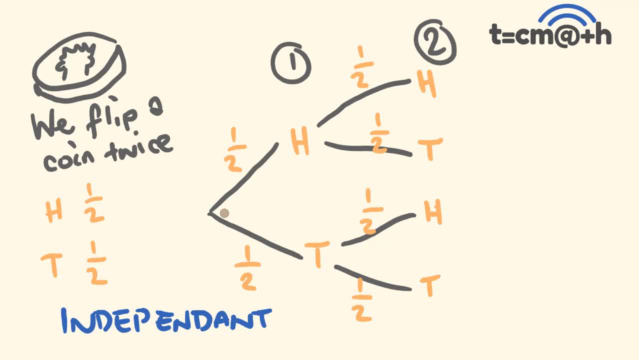 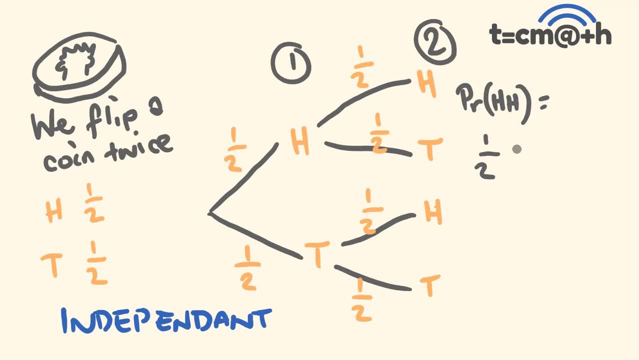 get a head here, and the probability getting the second one is also a half. Now this gets to a first rule of probability with multiple events and that's the product rule. Pretty much the probability of two or more events occurring together can be calculated. So two or more. 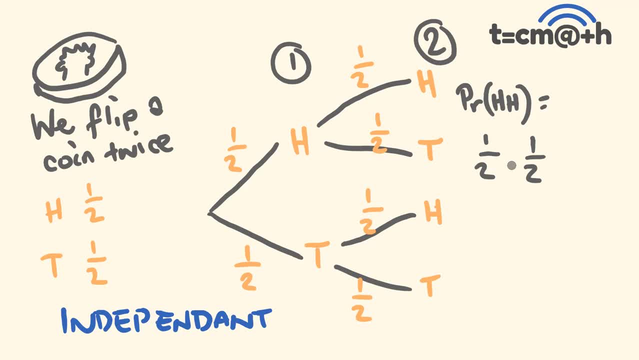 events getting a head and getting a head can be calculated simply by multiplying these individual probabilities. Okay, so the probability one times one is one. two times two is four. The probability of getting two heads is one in four. Okay, what about the probability of getting tails, tails and 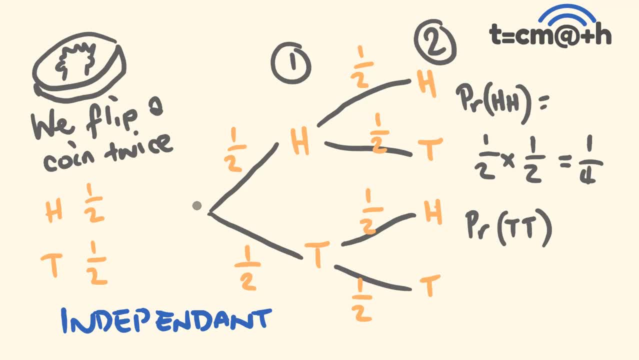 tails. You'll probably look at this and go: okay, it's the same sort of thing. The probability getting a tails is a half, the probability getting a tails is also a half, and so we're talking about this event, followed by this event. We're going to multiply these. This is a one in four chance. 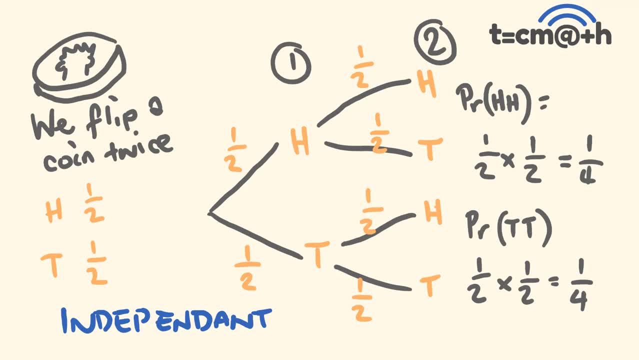 Okay, I'm just going to take this one step further and show you how to do it. So let's say, we've got a head here and we've got a tail here and we've got a tail here and we're going to do a different rule of this. I'll just give myself a bit of space here. 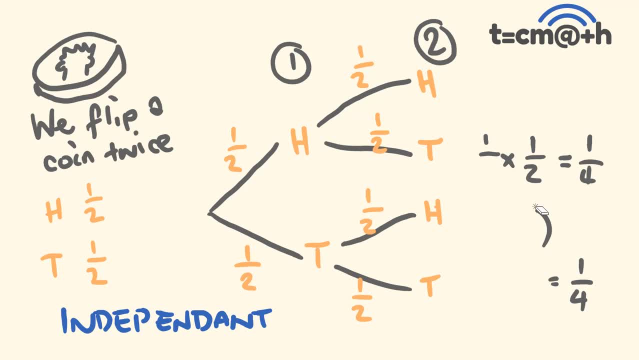 So I'm going to get rid of these two probabilities here and we're going to talk about a different thing that might occur. What about the probability of getting one head and one tail, but not necessarily in that order. It might be a tail and a head or a head and a tail, and you're going to see to do that. 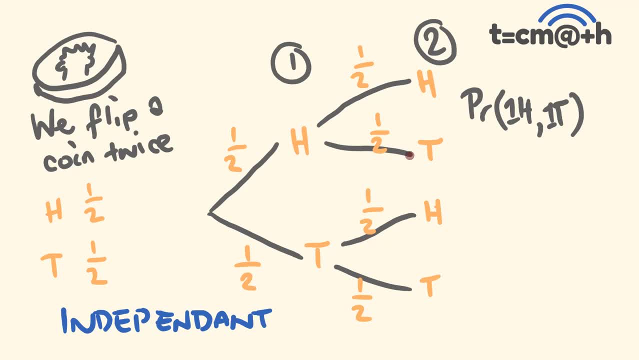 we actually have two different ways it can occur. We could, first off, get a head and then a tail, or we could get a tail and then a head. So I'm going to write both of these ones down. So, first off, if we go to the next one, we're going to get a head and then a tail. So I'm going to write both of. 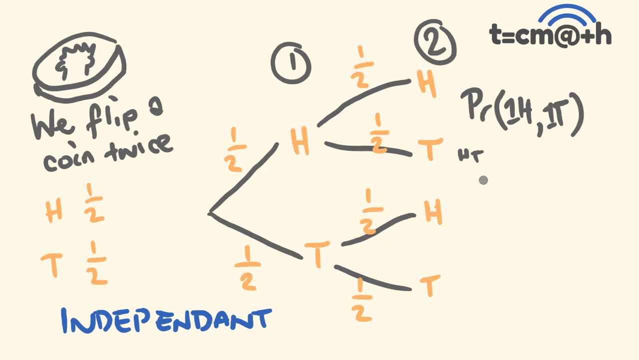 these ones down. So, first off, if we go to the next one, we're going to get a head and then a tail. The probability of getting that is a half of getting that first head and then a half. You might say, okay, we're going to multiply those because they're in a. you know that, particularly this event. 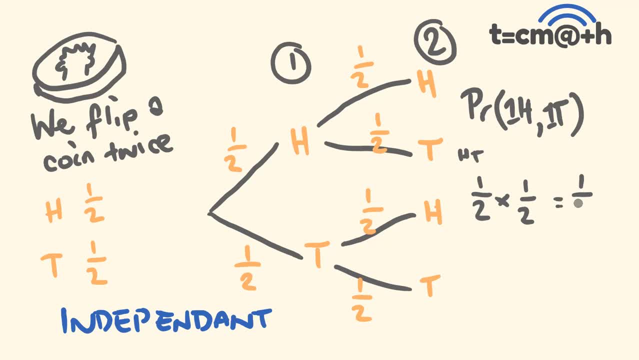 followed by this event. We're going to multiply these. This is a one in four chance of getting a head and a tail. The chance of getting a tail then a head is also a half times a half- Okay, a half times a half, which is equal to a quarter. So this gets to our second rule, when we're 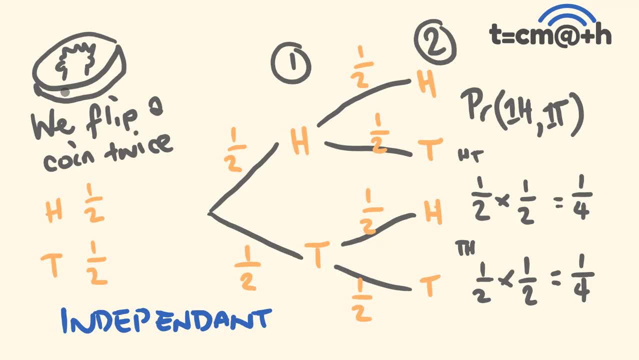 looking at multiple events and probability is this: If we're talking about two events that are mutually exclusive, that are not affecting one another, we're trying to find out the total probability, say, of something like with a tail and a head here, and there's a couple of different ways. 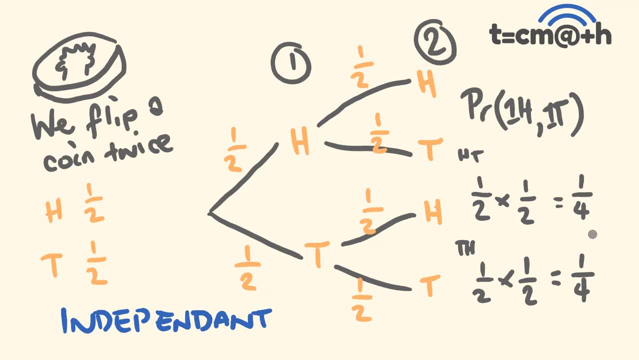 this can occur for our outcomes. What we do is we're going to add these. We're going to add a quarter and a quarter to get the total probability, because a head and a tail is the same as a tail and a head. So what's a quarter plus a quarter? You'd probably look 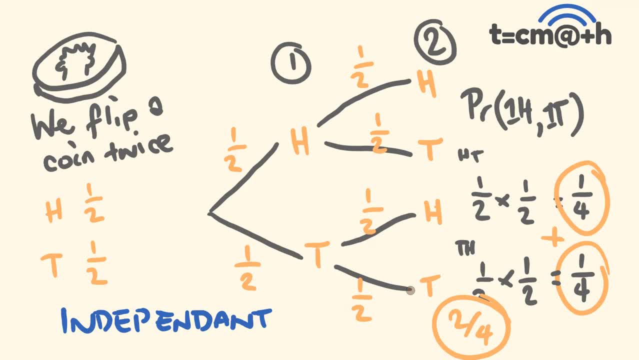 at it and say, okay, that's two quarters Okay, so the probability of that occurring is two quarters okay, or a half, So something to be aware of, Okay. so that's the product rule where we multiply these. if we're looking at something occurring in a line like that and if we've got something which is 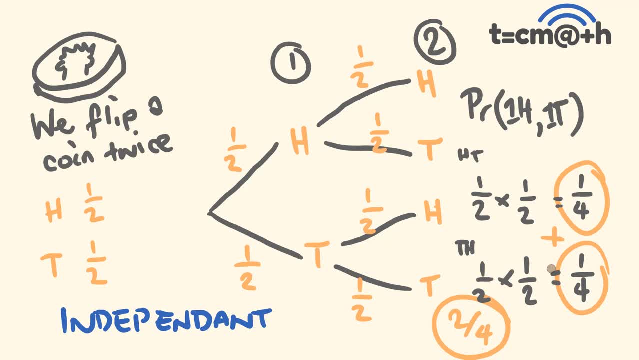 occurring, you know, and we're saying it's: uh, we want this and this occurring, we're going to add them together. Okay, that's the addition rule. So I'm going to go through another example and show you just a variation of this. All right, in this example, what we're going to have a look at is we: 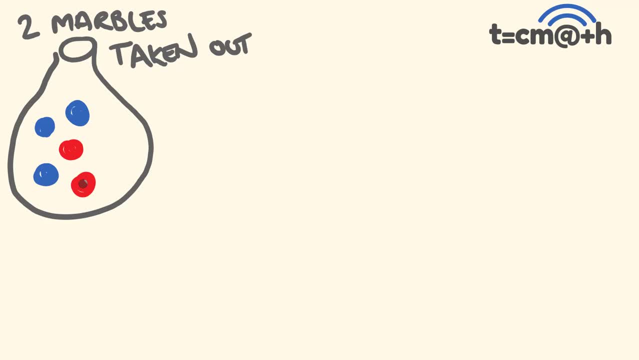 have a two quarter and a half. So we're going to add this and this occurring, and we're going to have a bag and it has three blue marbles and two red marbles and we're going to take two marbles out. Now we're going to work out also now what our different probabilities or different outcomes. 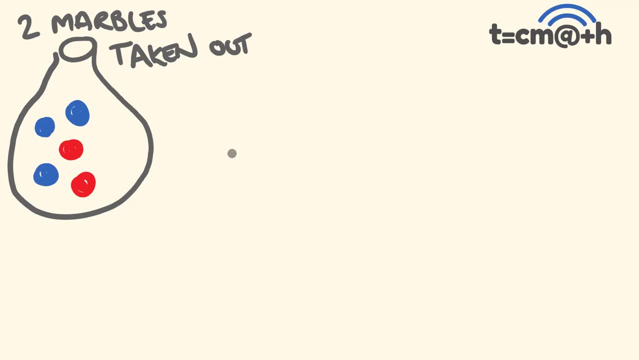 could be and the probabilities of those outcomes occurring. So, once again, let's draw up a tree diagram. So we have our first event where we're taking out the first marble. Okay, so the first marble you'll probably look at and say, okay, we could either end up with a blue marble or we could. 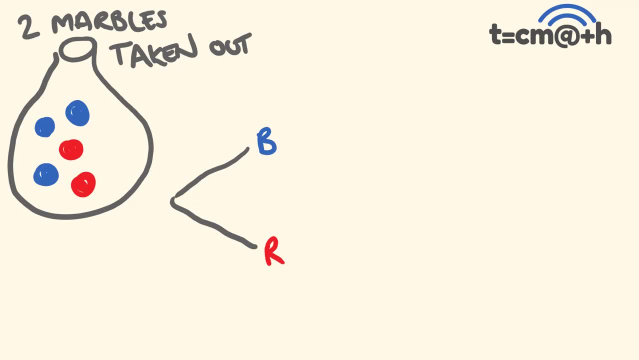 end up with a red marble. So we do that, then we're going to pull out the blue marble. We get rid of that, for instance, and then the next event, what we could do- is we might end up with a blue marble or a red marble, or for. 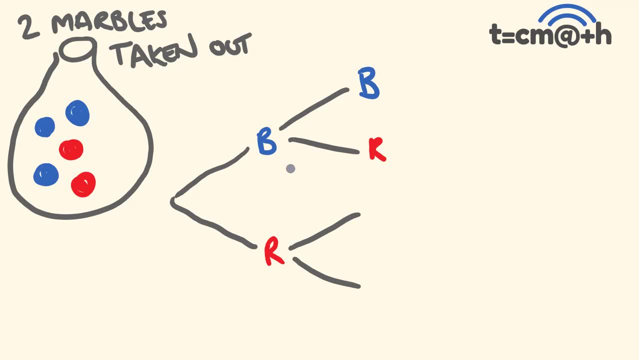 the. we might get a red one first. we could end up with a blue marble or a red marble. Okay, so let's have a bit of a look here about the various probabilities of each individual part here. Now, this is something to be very, very wary of, because the probability of each event 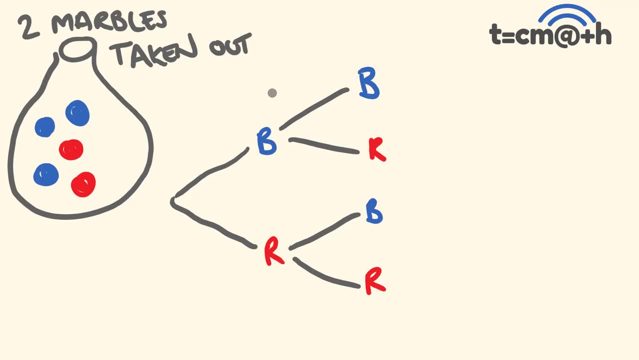 is not independent. Okay, each probability is, each particular event is not independent of the other. I'll show you what I mean by that. So say, for instance, I pull this first blue marble out, You can probably guess. okay, there's three blue marbles out of a total of five marbles For the reds there. 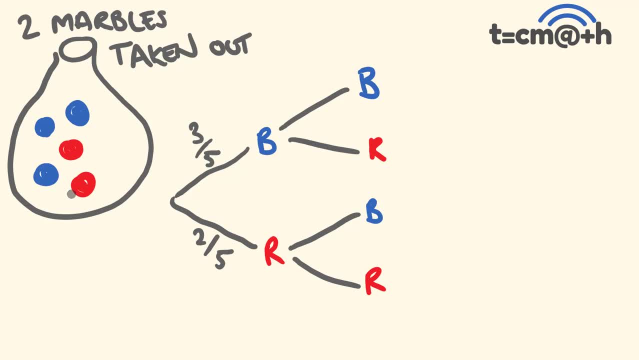 is two out of five. We have a two out of five chance of getting a red marble first. That's for our first removal. For the second one, what you might notice is this: if I was to remove, okay, we pick a blue marble out of it. Now, what's the actual probability getting a blue marble Now? because these are not. 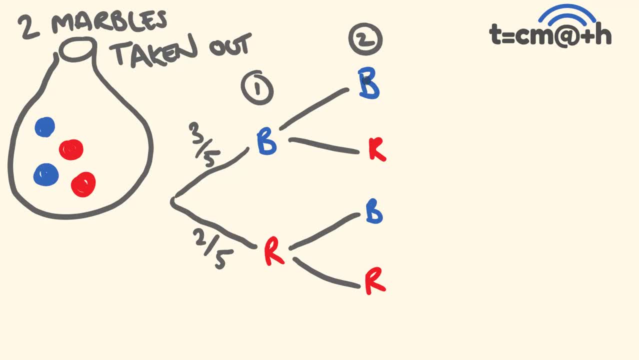 independent. they are dependent on one another. This actually now depends- the probability of this depends- on what happened here. We have two blue marbles now out of a possible four, and to get a red, we have two out of four. Okay, maybe that didn't happen and maybe what happened instead. 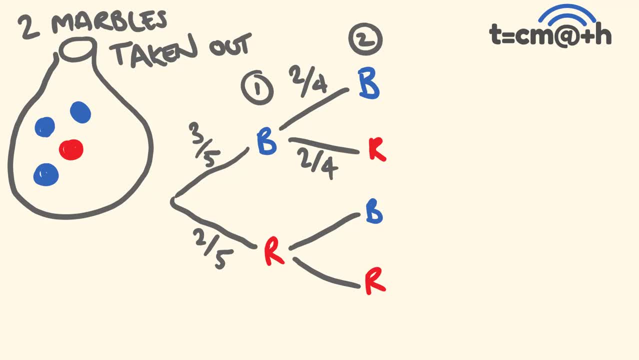 is, we went down here and we picked a red out first, so we got rid of a red. What's the probability of that happening so far? Well then, you probably have already got rid of one out of four, because last time something happened nowhere greater than five. So what we have right now is an additional. 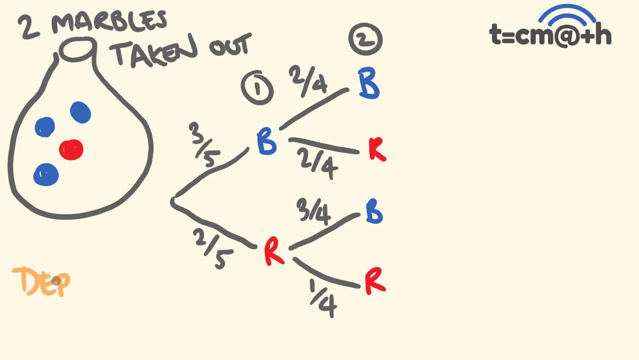 ா three out of four. The probability of getting a red is one out of four, and this is an example. I'll write that down. these are where we have different events that are dependent on each other. dependent, okay, and it's something to be really. 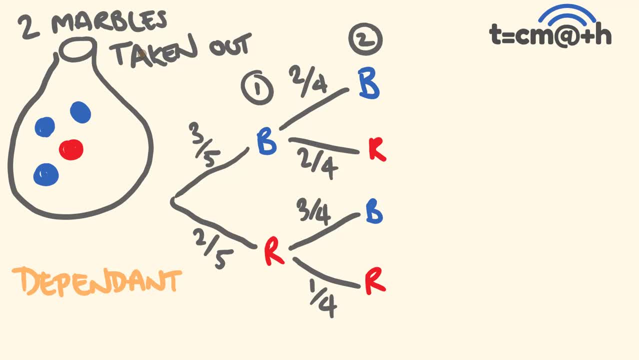 really aware of, because it changes these probabilities. as we go Bit of a hint here. what you might see is- occasionally you'll see this described: There's two tables. marbles are taken out without replacement. If they say they are replaced, what we're talking about is the 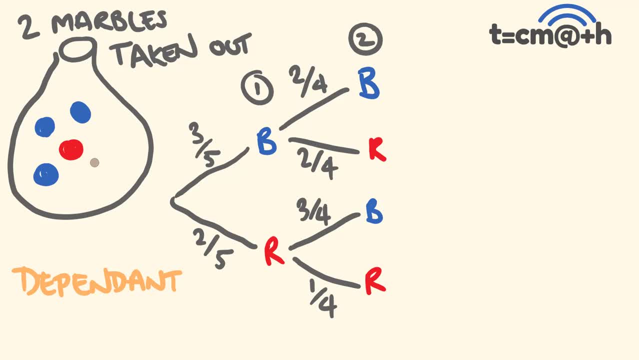 marbles get put back in, and what it would mean is that we would end up with a independent type scenario, okay, where we'd end up with still five marbles in here. so it wouldn't really affect these later ones and it wouldn't affect the probabilities here. so you'll probably notice here that we can. 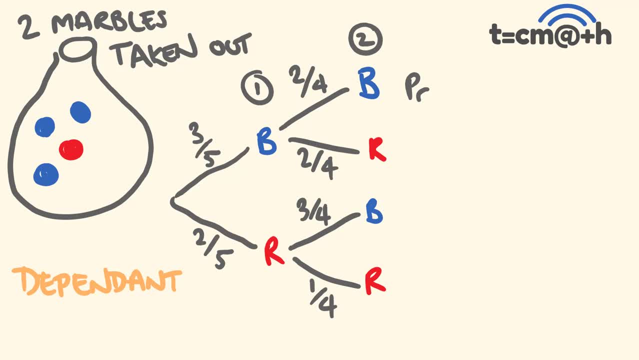 work out probabilities here. what's the probability of getting, uh, two blues, or i'm going to go through each one of these. what's the probability of getting a blue and a red? what's the probability of getting a red and a blue, red and a blue? what's the probability of getting a red and a red? 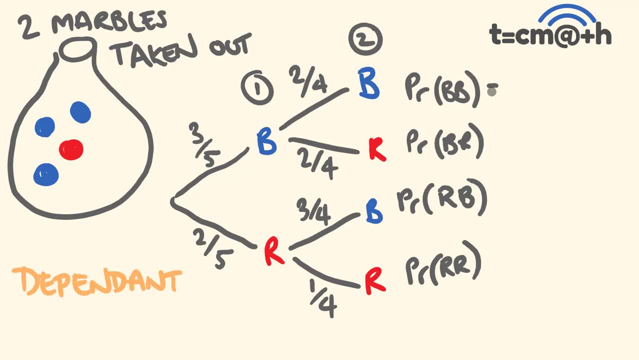 okay, let's have a quick look at these and these are all going to end up being product ones. we're going to multiply these. we go along the product. yeah, we got a three and five chance of getting the first blue. we have a two in four chance of getting the second blue. multiply these here. two. 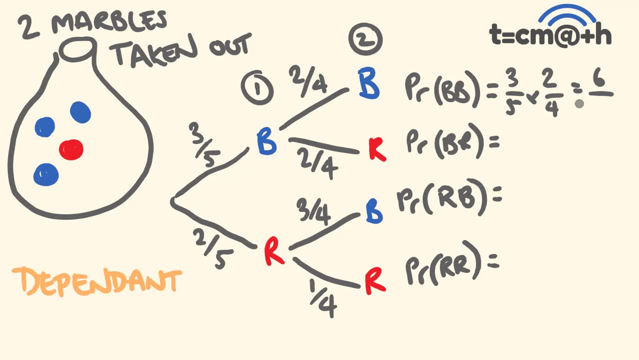 times three is equal to six. five times four is equal to twenty. you now, i know we could simplify this further- i'm going to leave that to you. i'm not going to do that right now because, let's face it, i'm going to run out of space if i do that. what about the? 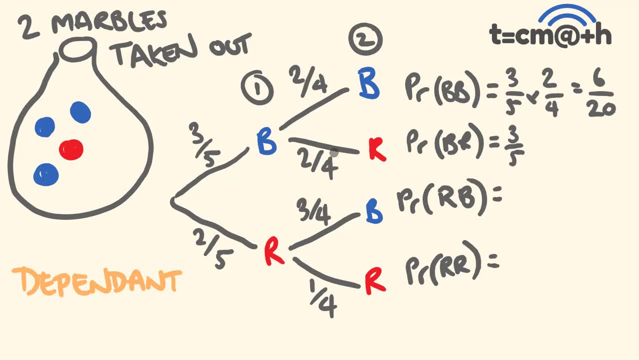 probability of getting a blue then a red. there's a three and a five chance of getting the blue, and to get this red here there's a two in four chance. so this also is a six and twenty probability, this one. here we have a two in five chance of getting a red first and then a blue. 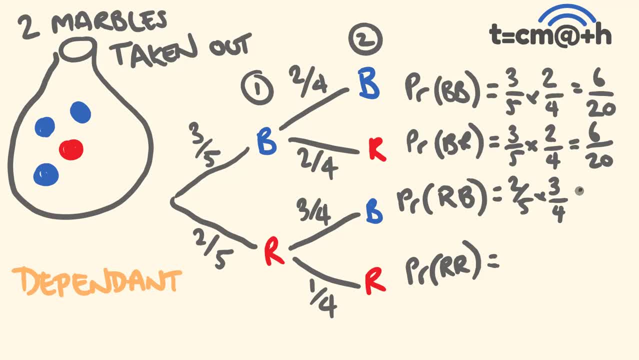 we have a three and four chance. we're going to multiply those. we end up with a- once again a six out of twenty probability to get two reds. there's a two in five chance at the start of actually getting the first red and then there's a one in four chance of getting that one, a second red, so two times one. 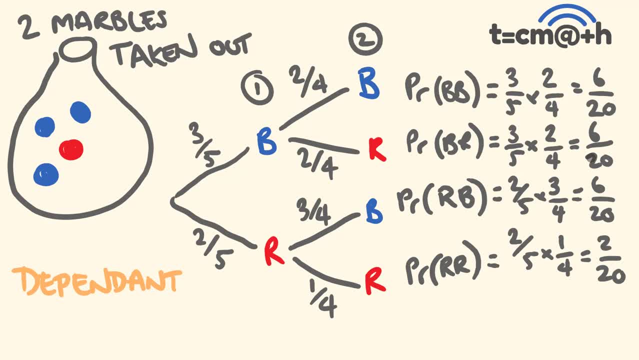 is two over twenty. you're going to notice, two plus six plus six plus six adds up to twenty. so all our probabilities are there and that's the product, uh, product rule in action there. now i might also say: okay, we can actually do this a little bit differently. and maybe i say, okay, what about a? 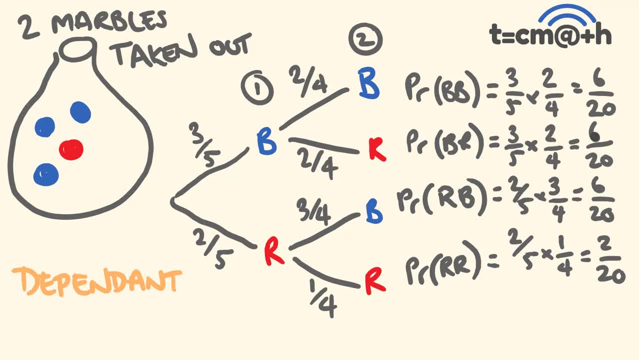 blue and a red, but not in any particular order. you go: okay, well, we'd have to add this: six out of twenty. okay, i'll even write this down here. i'm going to be struggling for space. anyway, i'm going to rub this out. i reckon i'll put it here. what's the probability of the one red? 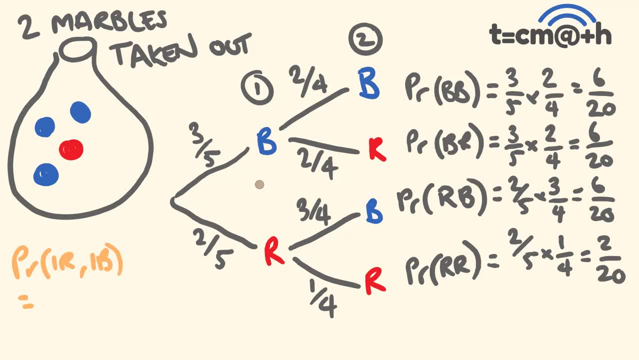 and one blue. you can sit there and go, okay. well, we've got two ways this could happen. we could get a blue and a red, which is a six out of twenty, and we've got a red and a blue, which is a six out of twenty, and we're going to add these. okay, this is a twelve out of twenty probability of getting a. 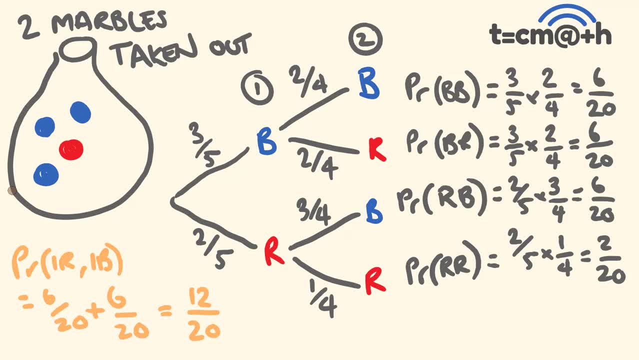 blue and a red. so this is a twelve out of twenty probability of getting a blue and a red. okay, so this is an example of a dependent event. okay, where an event actually changes the probabilities of each little part here and something to be wary of. what about one more example? okay, i'm going to 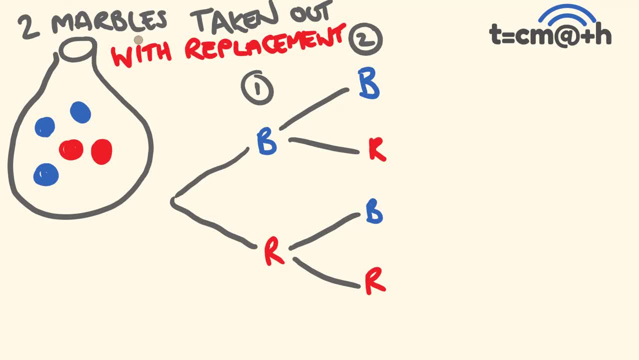 not vary this one up too much, because i think it maybe it's a good idea to do this at this stage. we're going to go two marbles taken out, same sort of bag. we have two reds and three blues, but this time with replacement. let's see what happens. okay, so if we take out the blue marble first, 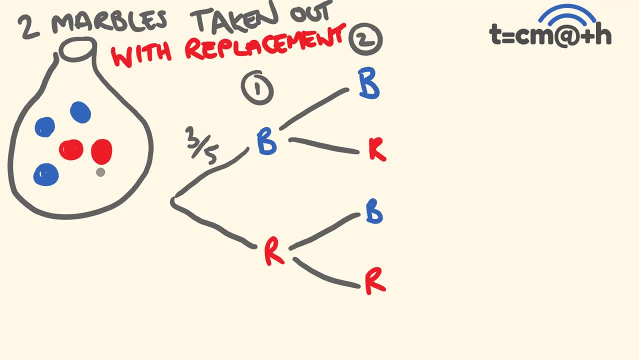 you have a three and five chance to get a red marble in the first drawing. you have a two in five chance. now imagine we uh, take this blue marble out. here we go, we're going to take it out, but it's going to get replaced, okay, so that means we're putting it back in. so i've taken it out, but now 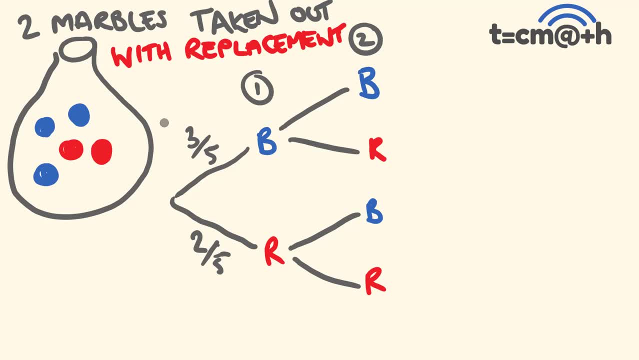 i'm putting it straight back in. so what's the chance now of getting a blue marble? and you go: okay, well, it's still actually three out of five, and to get a red is two out of five. okay, you're right, you're definitely going to have a three out of five against a blue marble. so this is the 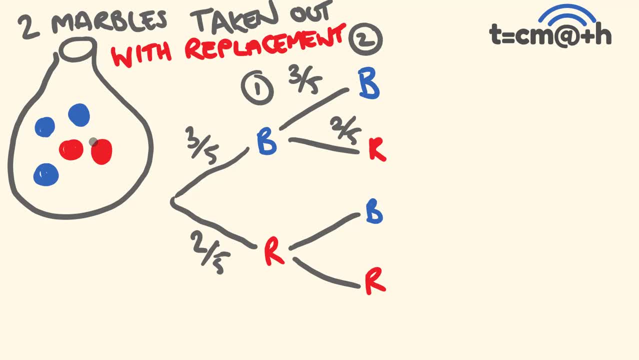 last thing that we show as two out of five, and what we're doing here is, if your temperature actually goes up or your temperature is pushed up, that'll get the sheer advantage of having it all the way down. we're going to create the next elaborate effect to it, so we're going to start with a single red marble again. 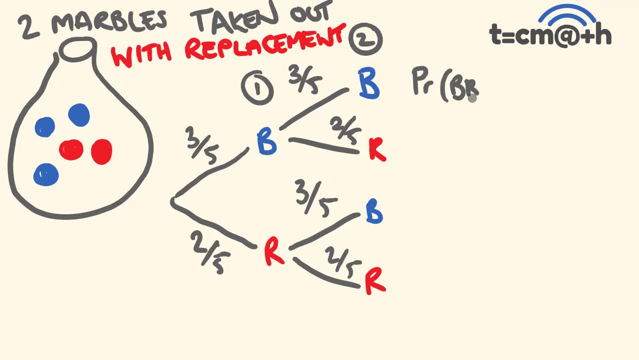 and what's going to happen is i'm going to create a red marble. this is going to be a more intellectual'll show you the installation. you know when you're organise a multi- Napoleon, which is going to be 3 times 3, is 9 over 25.. 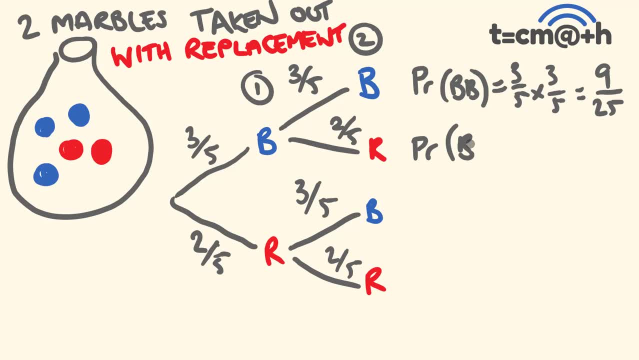 We've got a probability of getting, say, a blue and a red. A blue and a red is going to be equal to 3 out of 5 times 2 out of 5, which is going to be 6 out of 25.. 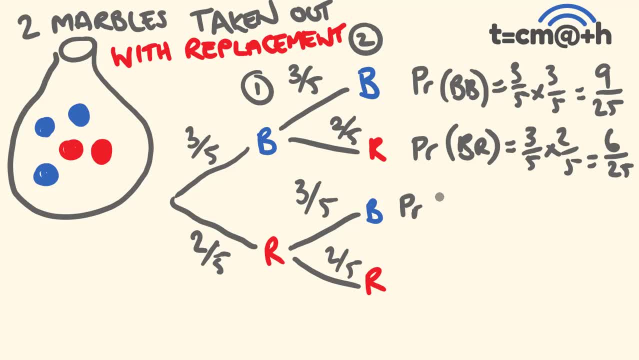 Okay, notice the probabilities are all of a sudden different. The probabilities of getting a red and a blue is equal to 2 out of 5 times 3 out of 5.. 2 out of 5 times 3 out of 5.. 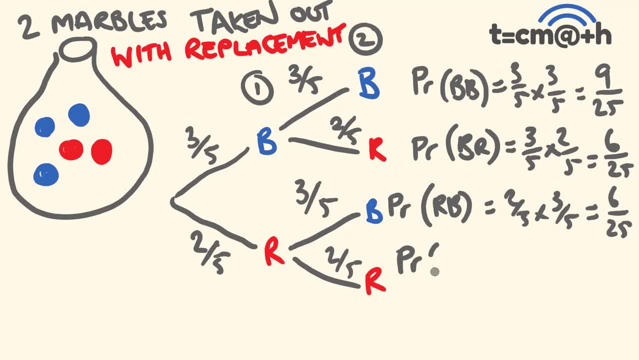 Which is going to be equal to 6 out of 25.. The probability of getting a red and a red is equal to 2 out of 5 times 2 out of 5,, which is going to be 4 out of 25.. 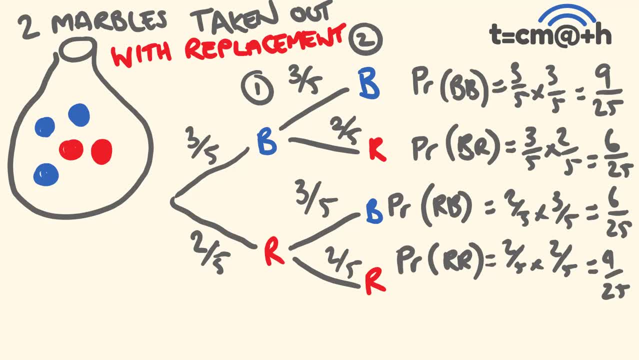 So be really, really careful of these. when you do these, If it's a replacement, you're going to treat it differently to if it's not replaced, okay. So you know you can actually now say, okay, what's the probability. 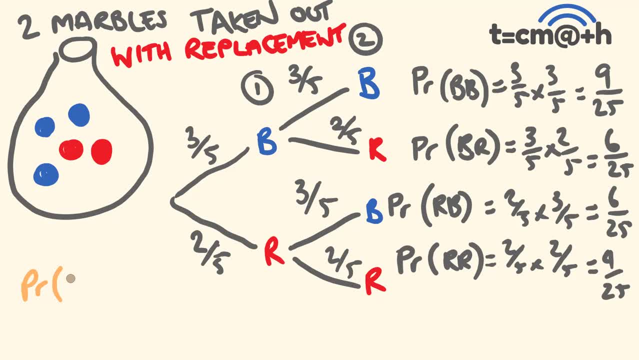 You can already say what's the probability. The probability of 2 blues or 2 reds is maybe the probability of at least 1 blue. What's the probability of this? Well, this one has at least 1 blue. This one has at least 1 blue. 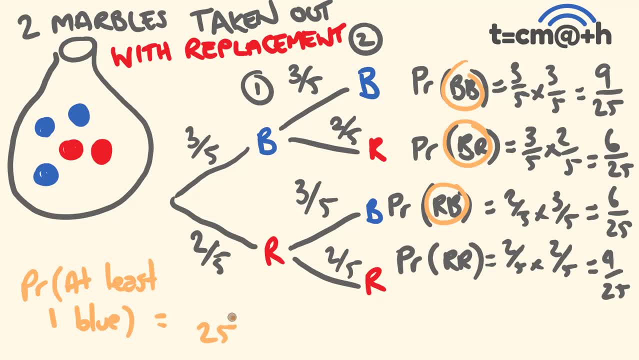 This one has at least 1 blue. It's out of 25 because we're going to add all these together. So 25,, 25,, 25, the denominator is staying the same. 9 plus 6 plus 6 is 12.. 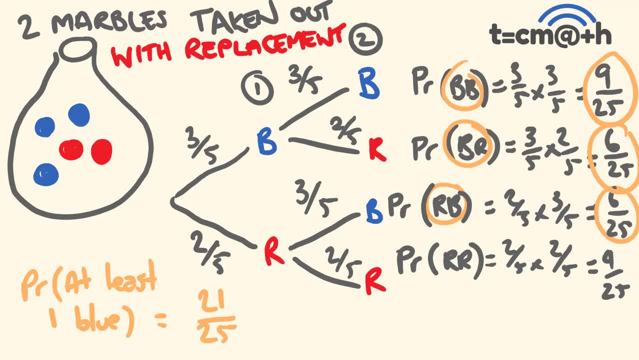 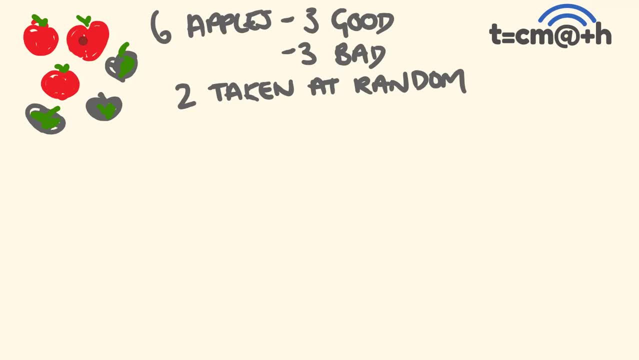 We have 21.. It's 21 out of 25 probability. Tell you what we'll do. one more Okay, in this example, what we're going to have a look at is a scenario where we have 6 apples where 3 of them are good and 3 of them are bad. 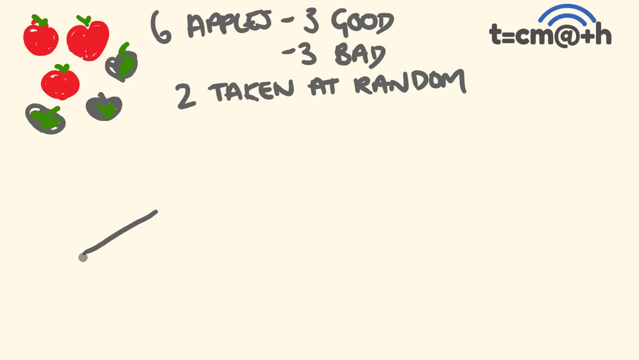 And we're going to take 2 out at random. Okay, so let's draw up our tree here. We have good bad. That's our first one. We have good bad, good bad. I reckon you should give this a go without waiting for me, by the way. 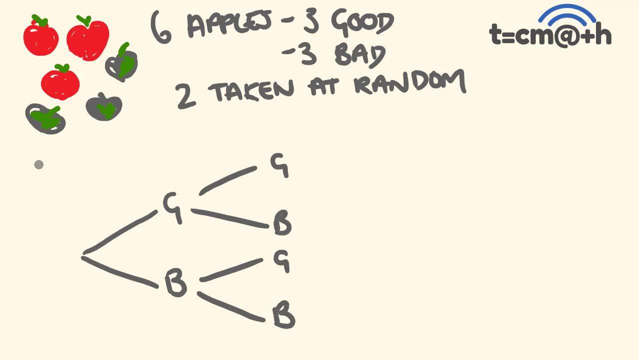 We're going to take these out at random And remember we're not actually putting them together, We're going to come back. There is no replacement. So what I recommend you go through first. can you work out the probabilities of each of these particular outcomes? 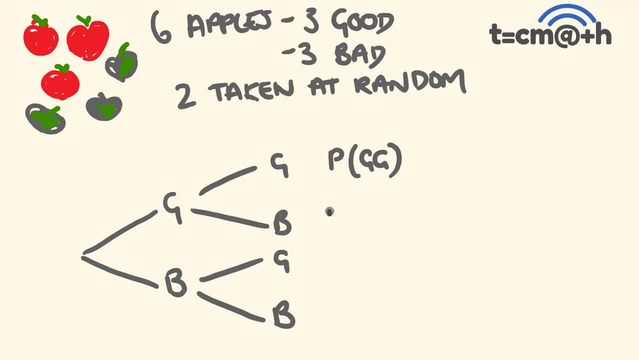 of getting a probability of getting a good good, the probability of getting a good bad, the probability of getting a bad good and the probability of getting a bad bad, And I'll just leave that one. We'll see how we go with those ones. 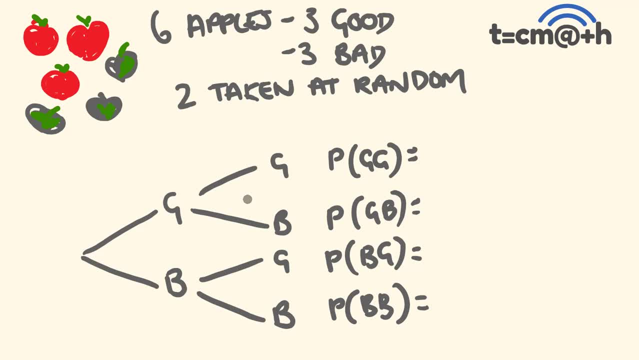 Go for it. So first off, go through and work out your probabilities of each particular event and then go from there Using those product rules. Okay, so give it a fly. Hopefully you did all right. Okay, the probability of getting a good apple to start off with is three out of six or a half. 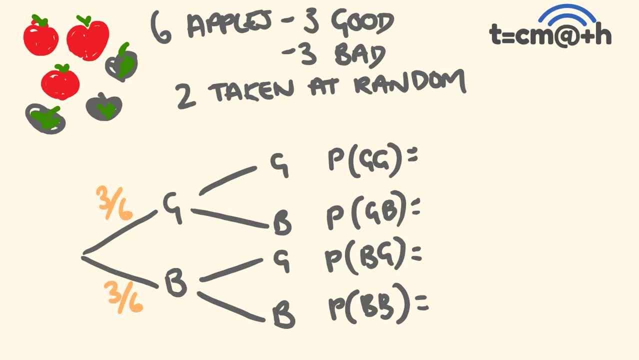 It's three out of six. here as well, If you choose a good apple first, I'm just going to say: we choose one of these, We'll get rid of it. So what's our probability now of getting a good apple? You might say, okay, it's two out of five. 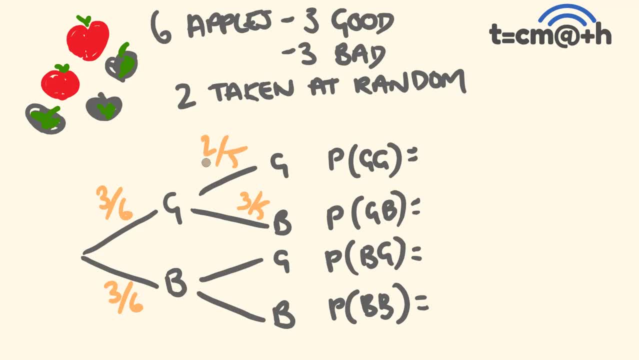 The probability of getting a bad apple is three out of five, Because these are actually dependent, particular dependent events here. Okay, well, maybe that didn't happen, Maybe my apple was okay And there it is, And instead what we did is we took a bad apple out first. 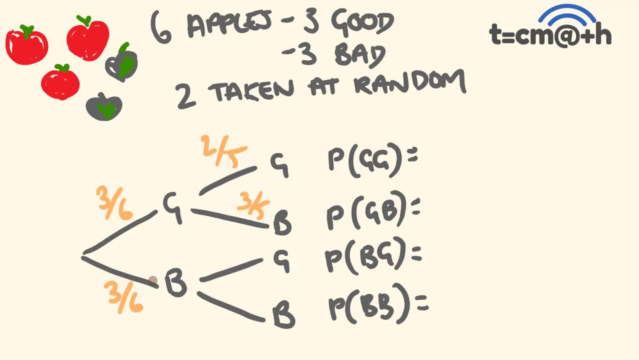 Okay, let's have a look at what happens here. You know, the probability of getting a good apple is now going to be three out of five. We have three good apples out of five apples. The probability of getting a bad apple is going to be two out of five. 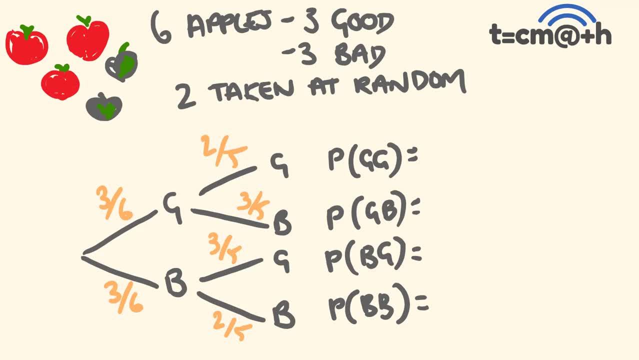 Okay, what's our different probabilities Here? probably, getting two good apples is three out of six times two out of five. We're just following up that pathway there: Three, twos of six, six, fives of 30. What's the probability of getting a good and a bad? 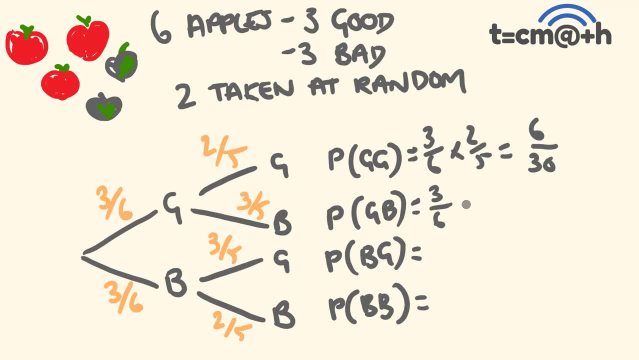 You might go. okay, that's a three out of six times three out of five, which is going to be three, threes and nine out of 30. The probability of getting a bad than a good. We have Three out of six times three out of five.